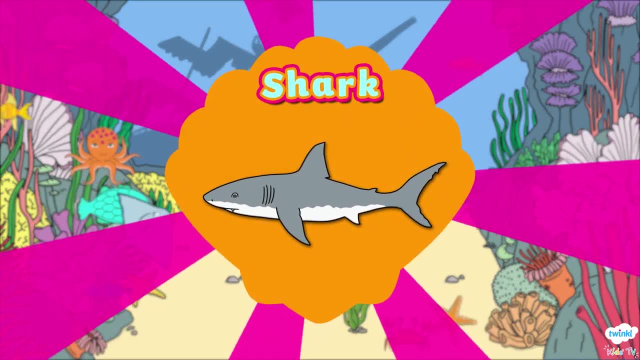 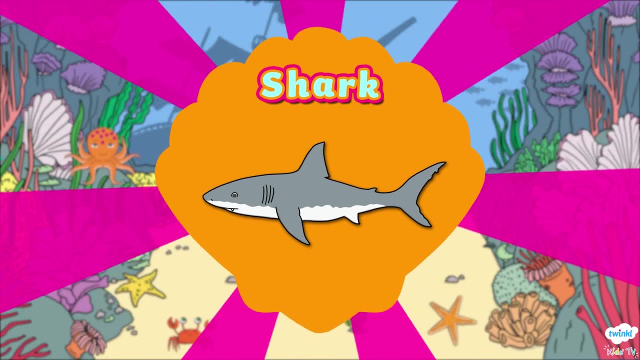 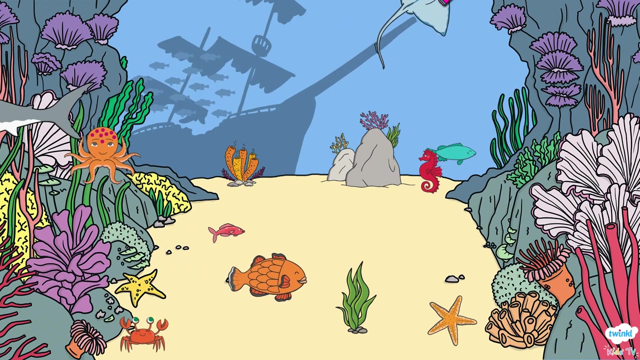 You got it: It's a shark. There are lots of different sharks in all shapes and sizes, but the biggest is the whale shark. Now for our next find. I spy with my little eye an animal that has five pointed arms and likes to live on the rocks at the bottom of the sea. 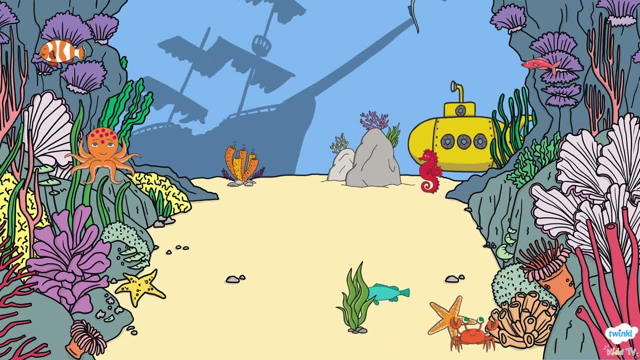 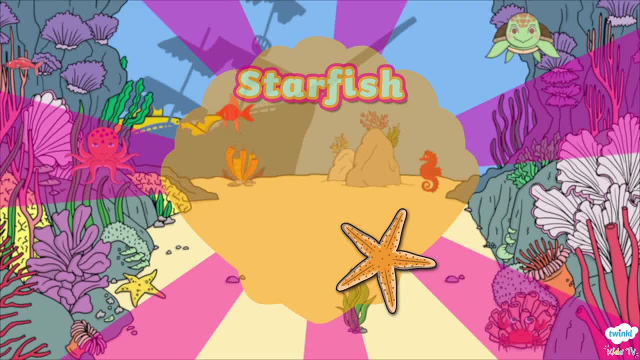 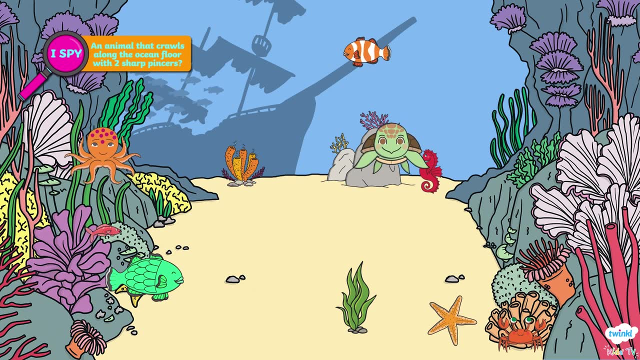 What could it be? Have you found it? Well done, It's a starfish. What's up next? I spy with my little eye an animal that crawls along the ocean floor with two sharp pincers. Can you see it? 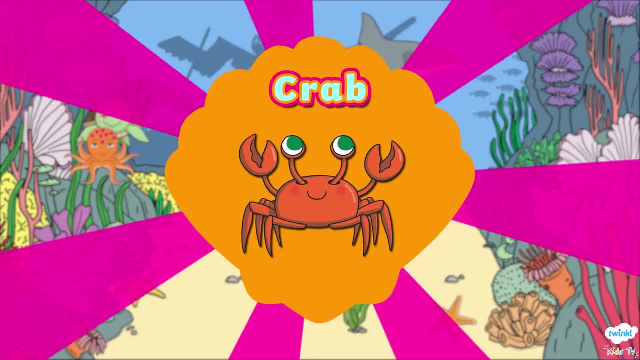 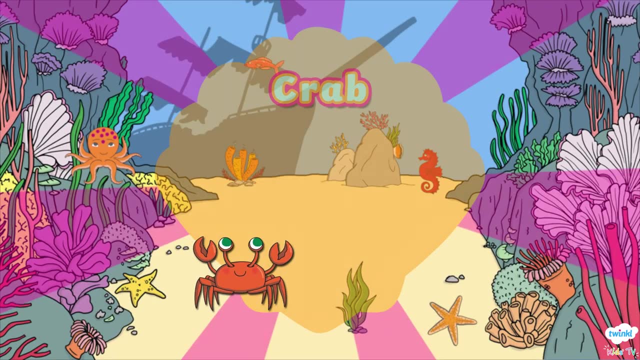 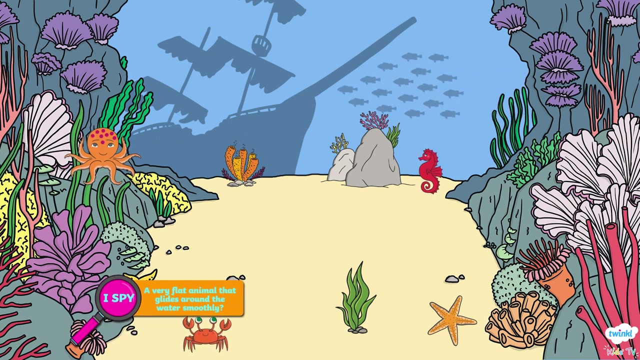 Great work, It's a crab. Crabs are actually crustaceans, Which means they have a hard shell. Great job. Now it's time for another. I spy a very flat animal that glides around the water so smoothly. What do you think it could be? 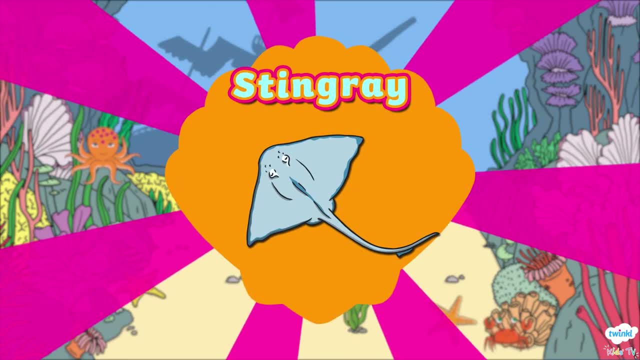 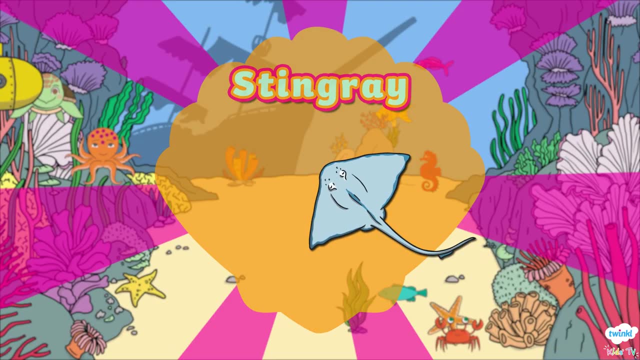 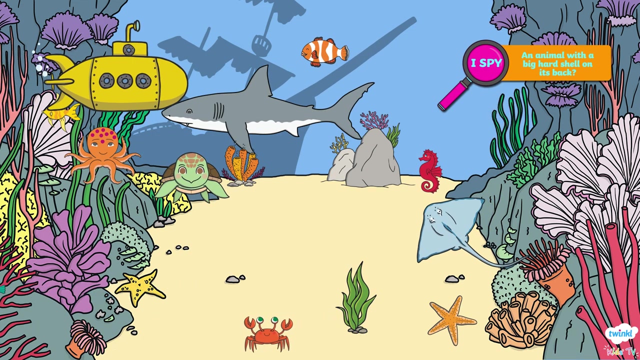 You've got it: It's a stingray. Stingrays actually have no bones, which is why they are so flat and smooth. Now, what can we see swimming in the sea? I spy with my little eye an animal with a big, hard shell on its back. 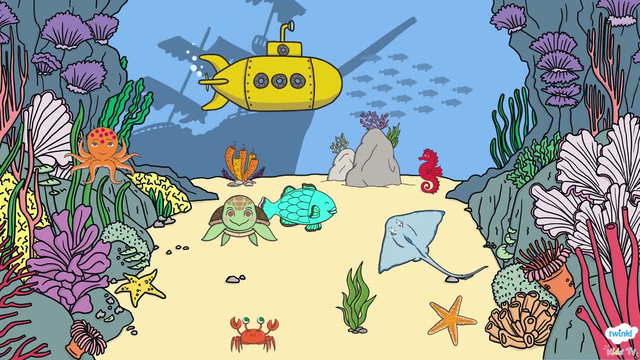 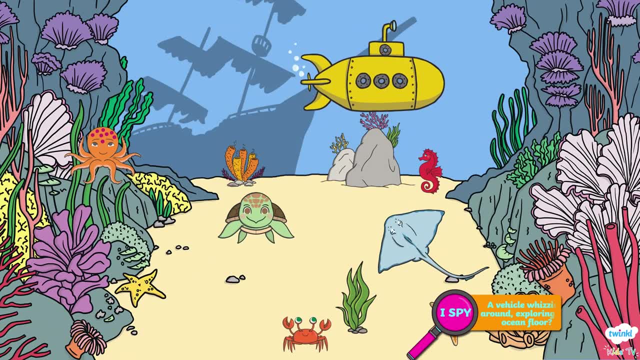 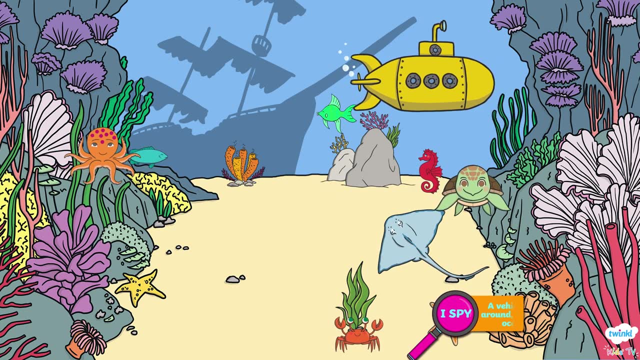 Do you know what it could be? You've found it: It's a sea turtle. Next up, I spy a vehicle whizzing around the water exploring the ocean floor. What could this be? Can you see it? It's a submarine. 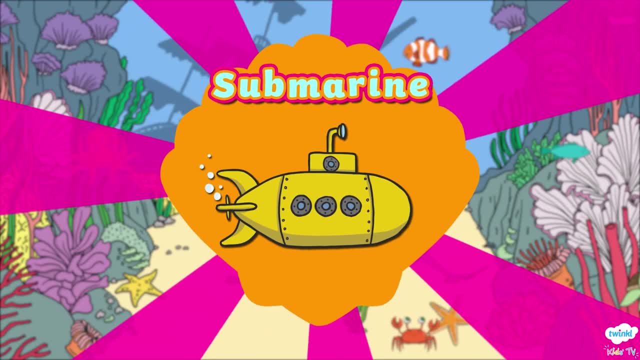 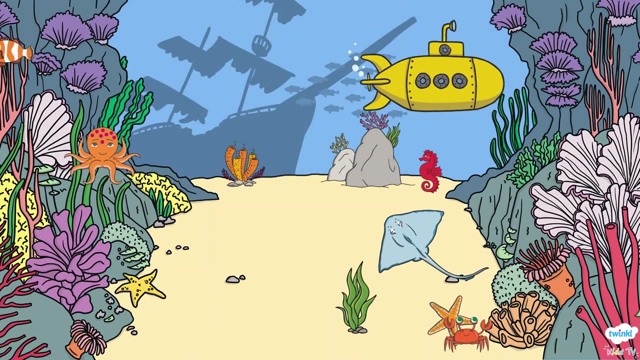 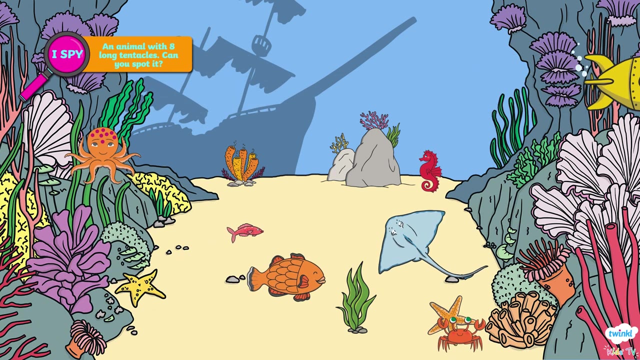 Submarines can go all the way underwater for us to explore all the fantastic things that live under the sea. What else do we have here? I spy an animal with eight long tentacles. Do you know what it could be? Can you spot it? 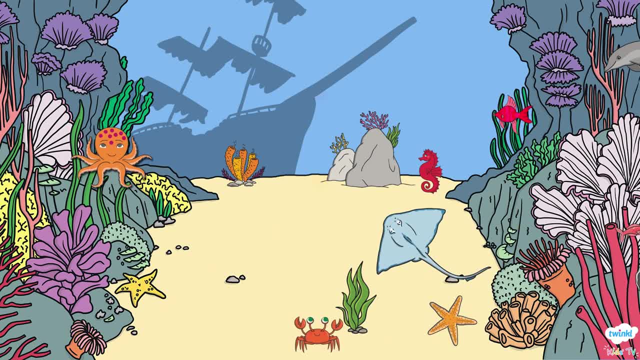 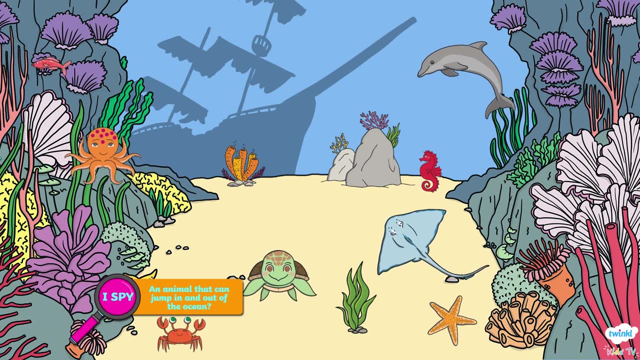 You've found it Well done. It's an octopus. Now for our next ocean, find I spy, an animal that can jump in and out of the ocean with ease, and it might even give you a smile. What do you think it could be?